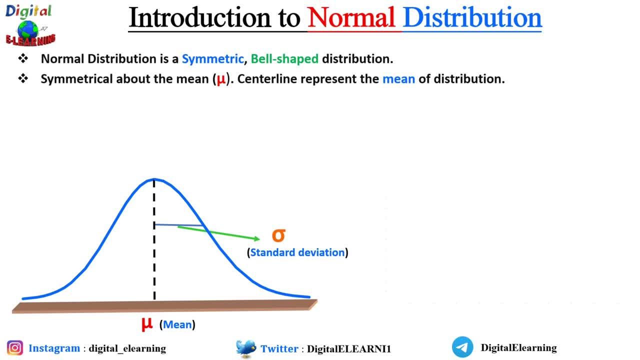 and this represents the standard deviation, that is, the distance from the mean. It extends from minus infinity to plus infinity. So the two tails that we have at the end of the normal distribution. it extends to infinity and never touches the horizontal axis. The property of the normal distribution is that it is a non-linear distribution. 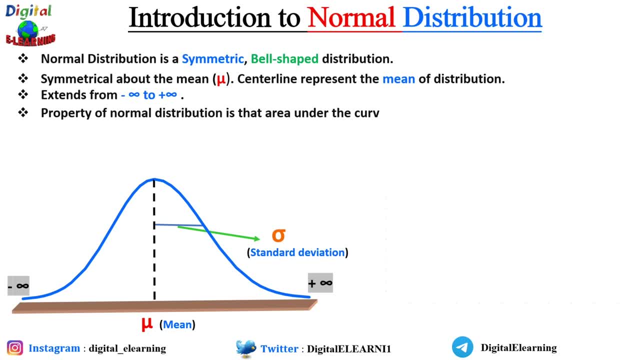 The property of the normal distribution is that the area under the curve, that is, the total area under the curve, is one and half of it is 0.5 and 0.5. so no matter what is the value of your mean, mu and sigma standard deviation, the total area under the curve remains one. 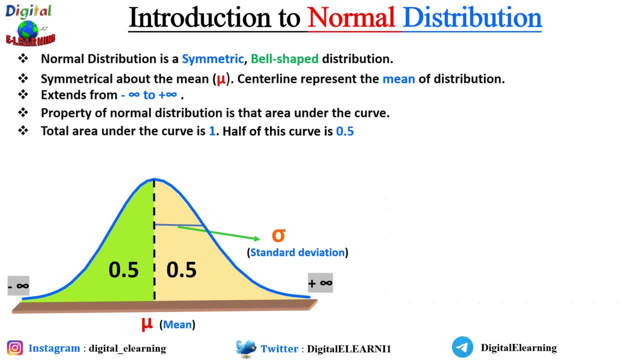 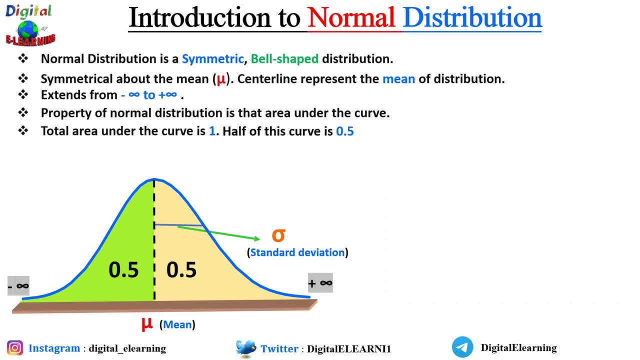 This curve has a single peak, meaning it is unimodal and not bi-unimodal. Because it is symmetric about the center, its mean, median and mode are the same values. Because it is symmetric about the center, its mean, median and mode are the same values. 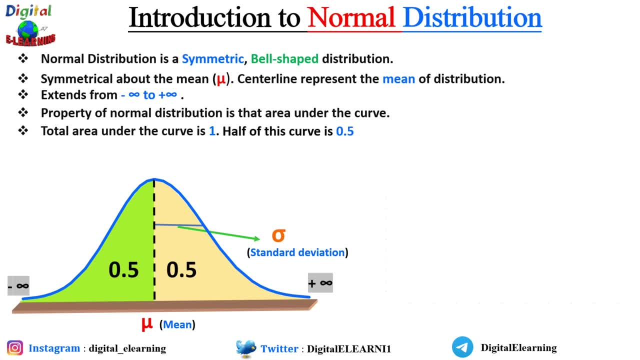 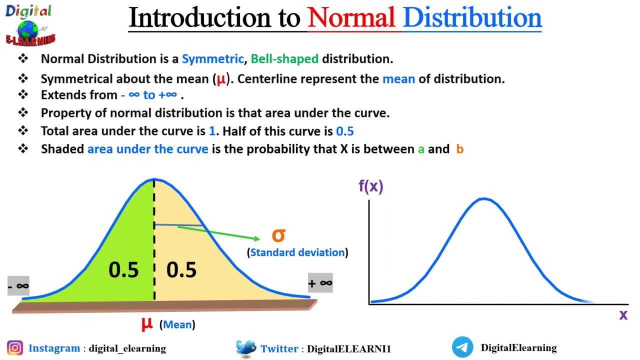 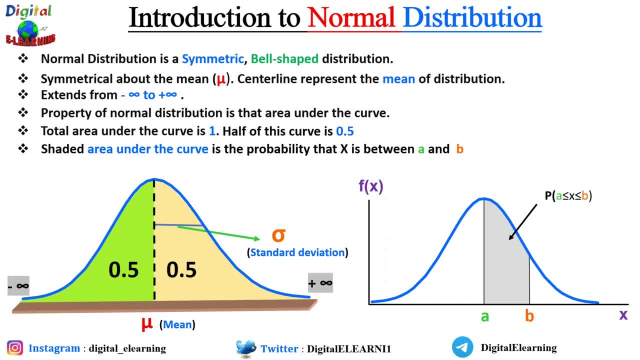 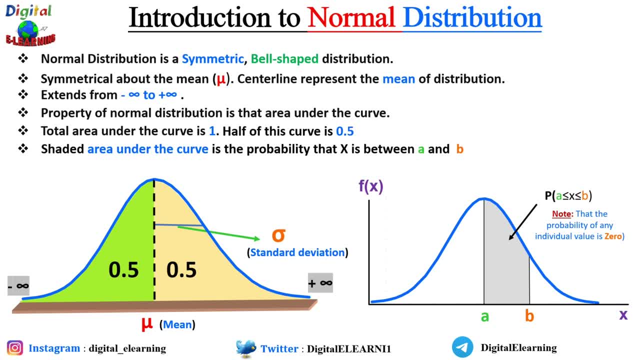 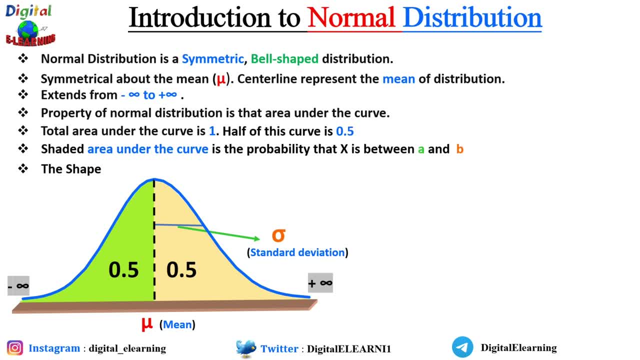 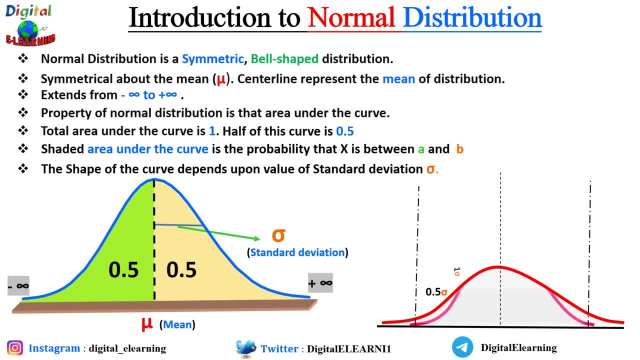 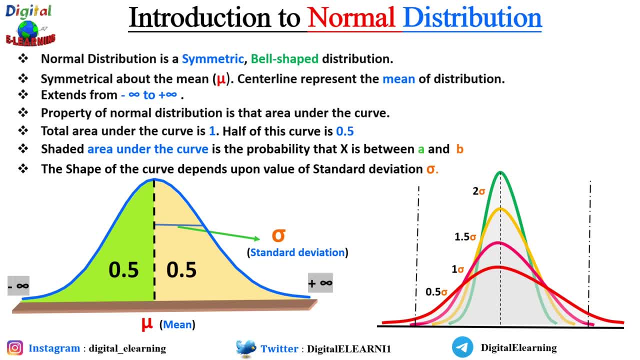 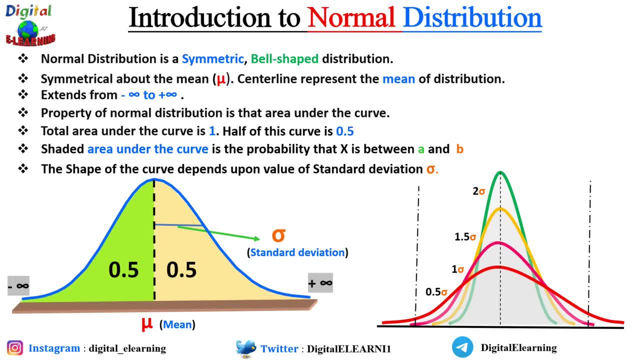 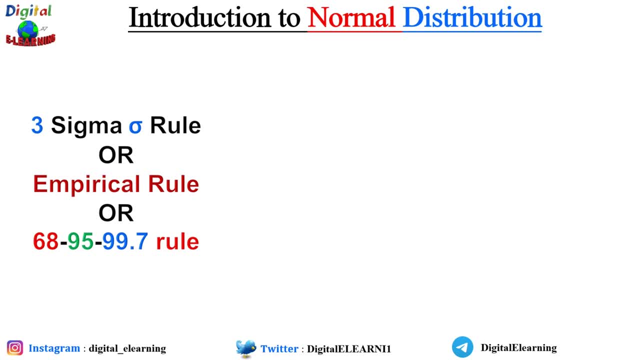 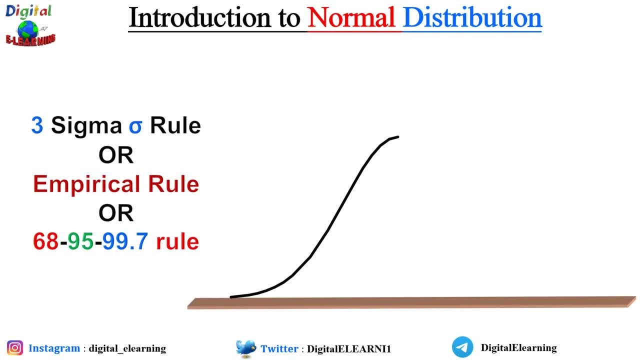 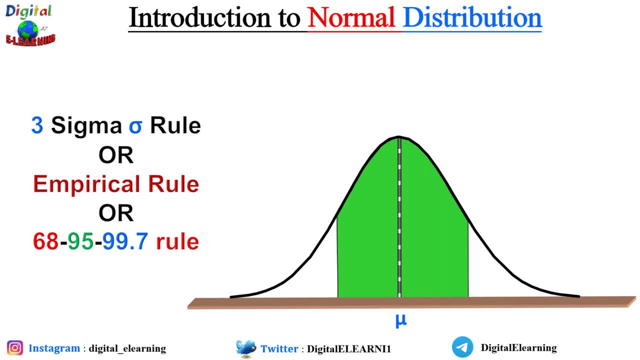 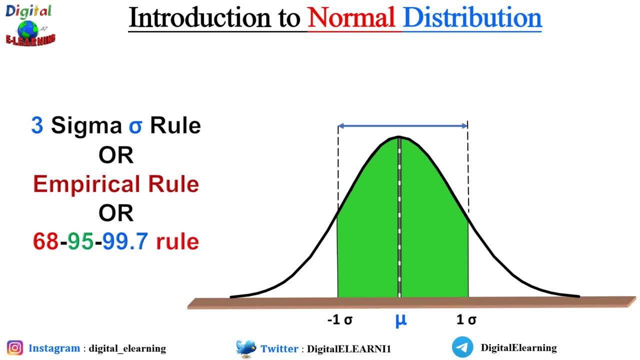 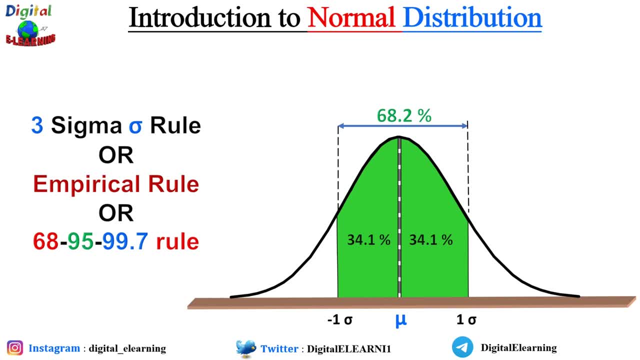 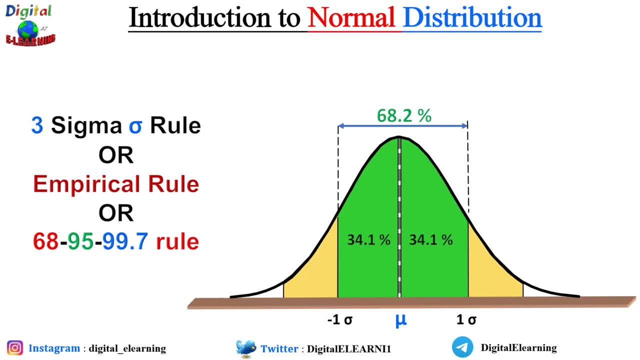 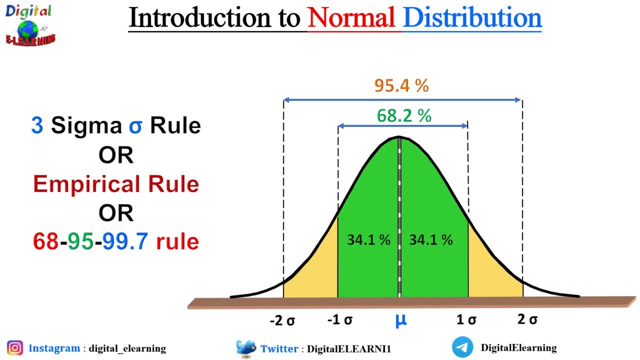 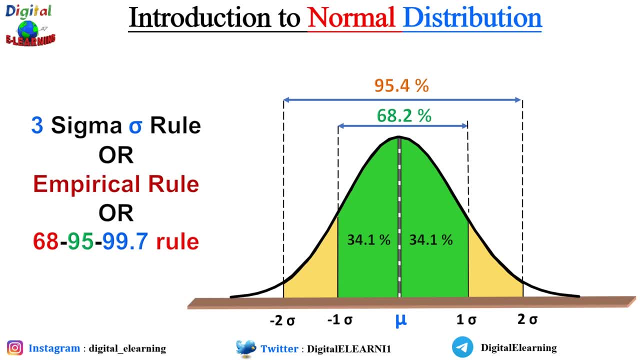 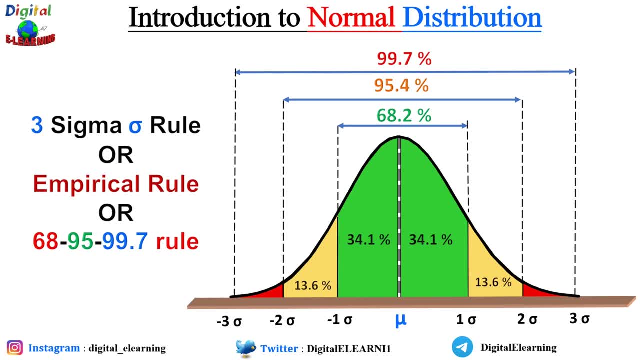 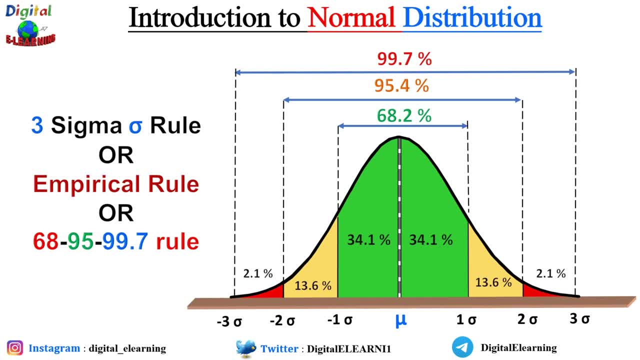 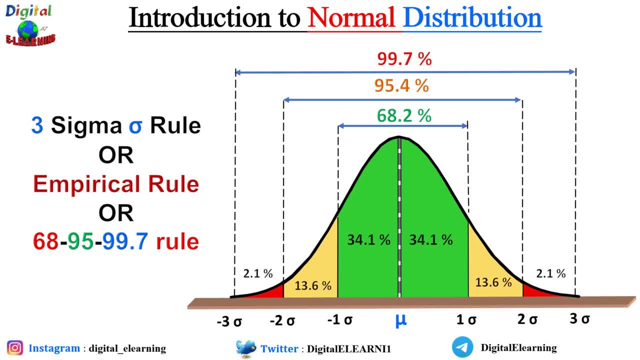 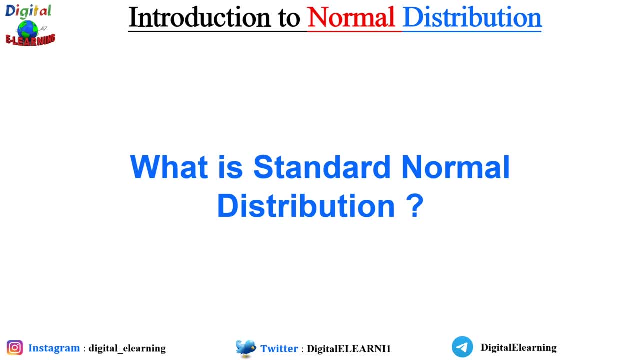 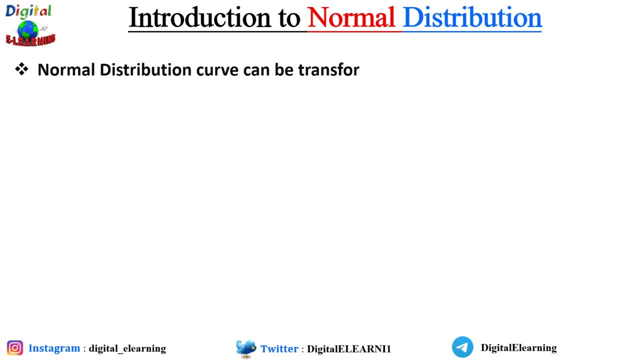 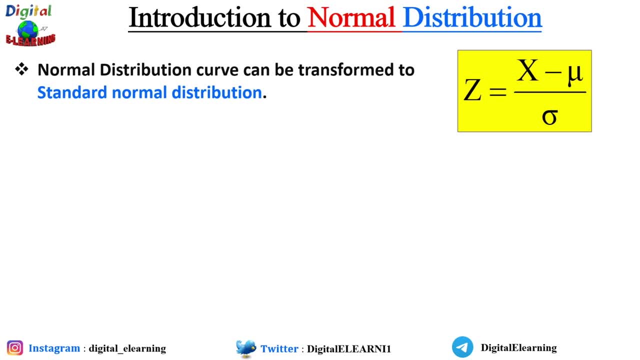 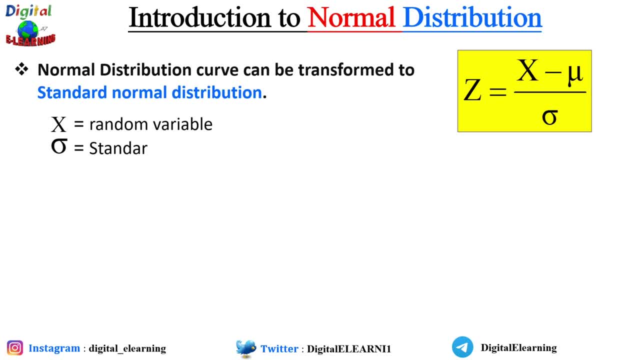 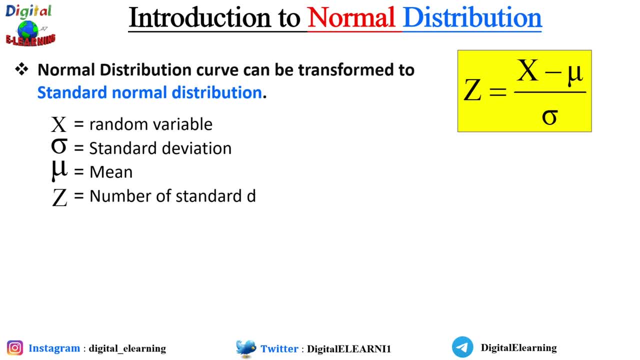 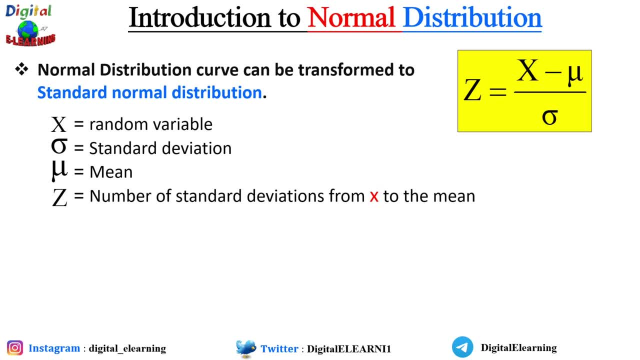 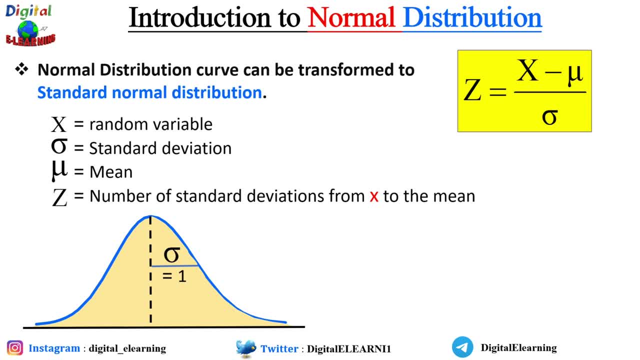 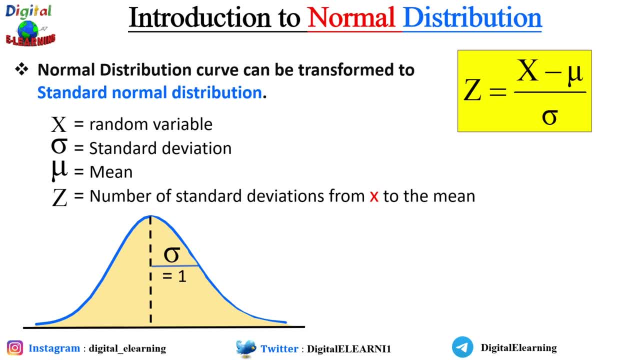 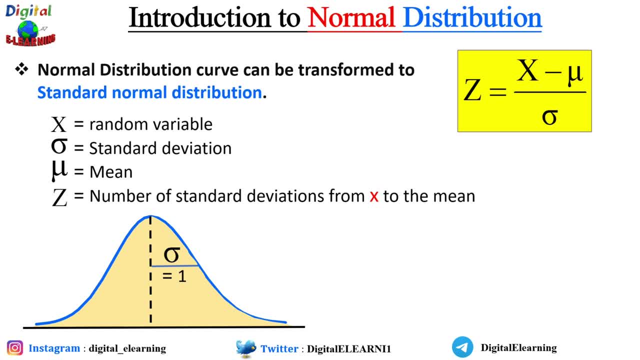 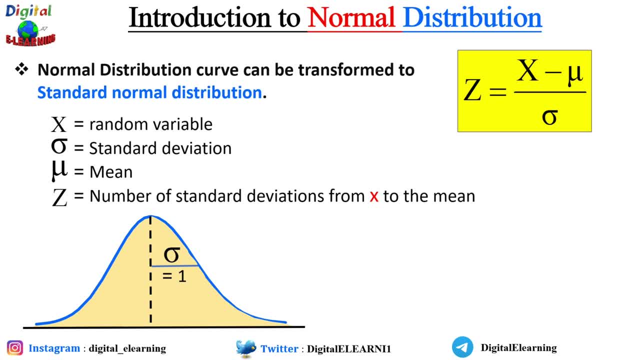 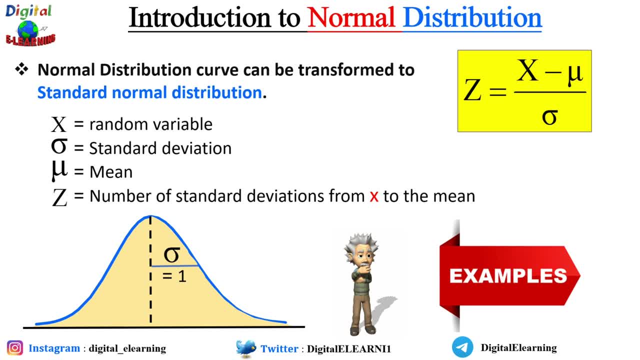 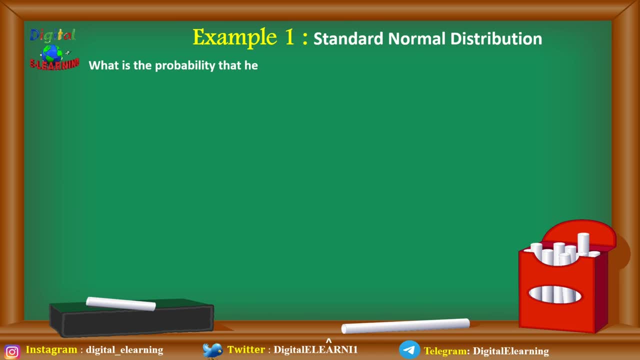 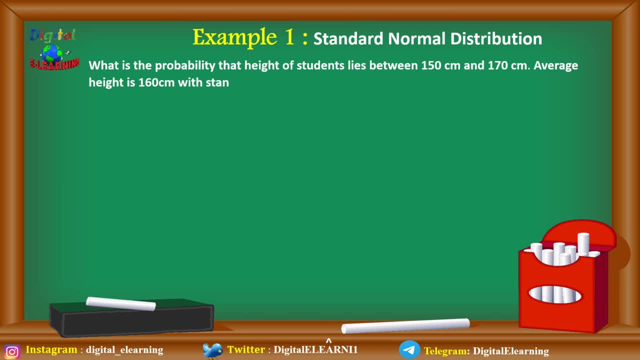 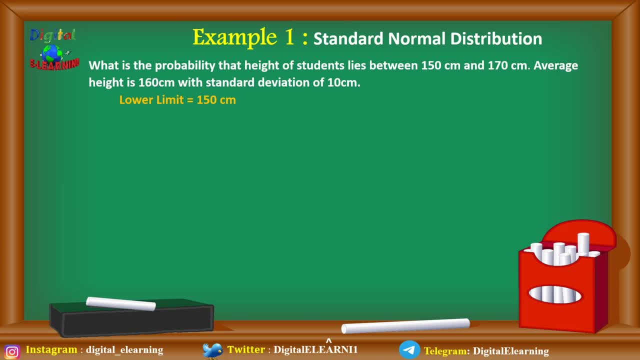 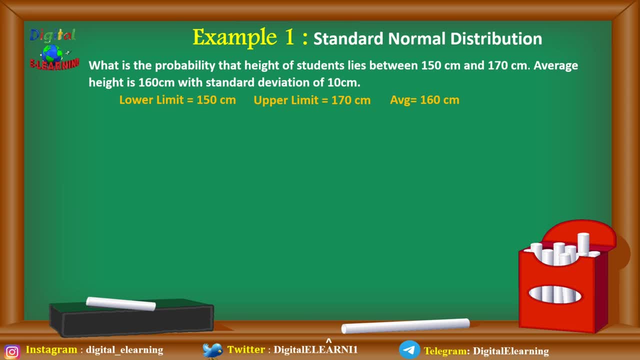 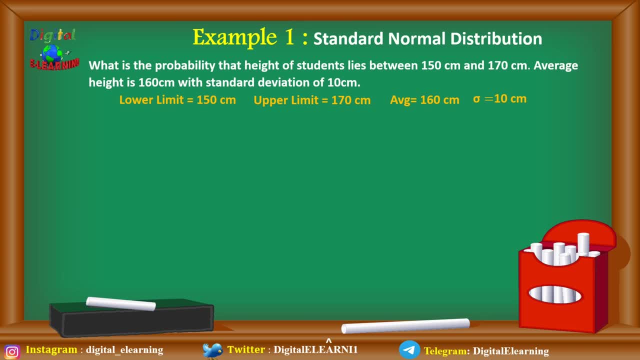 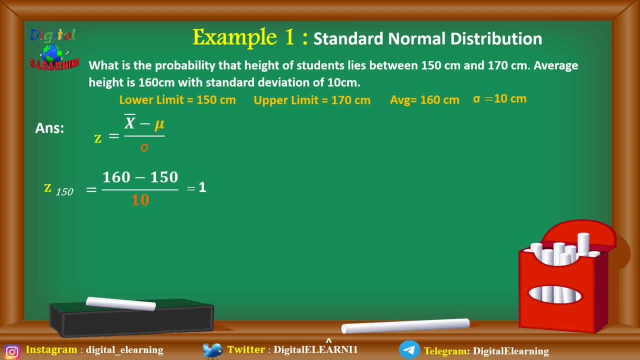 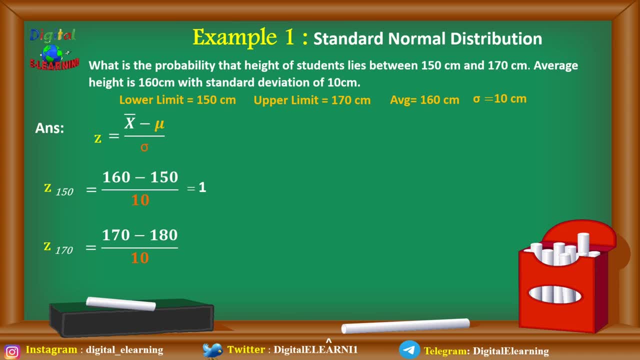 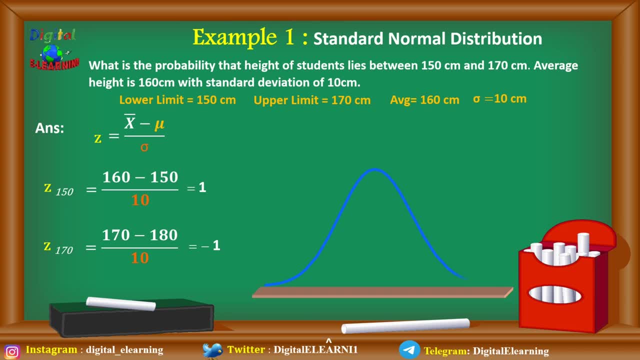 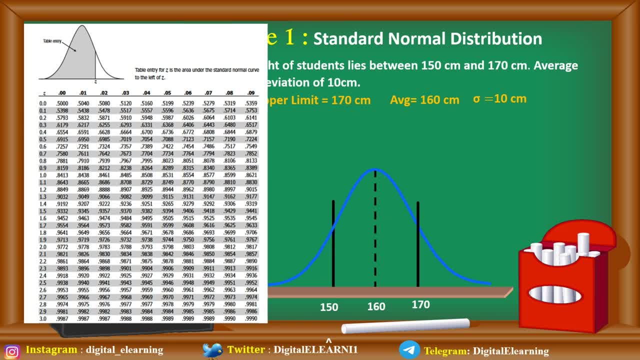 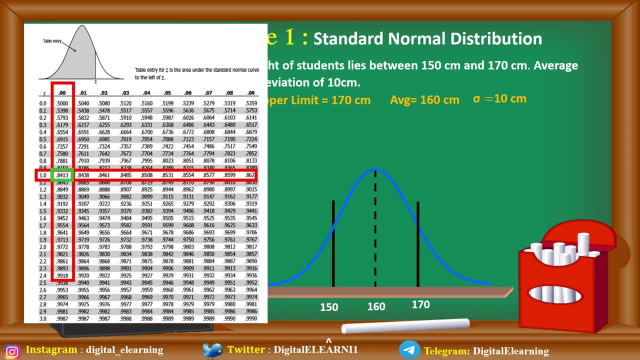 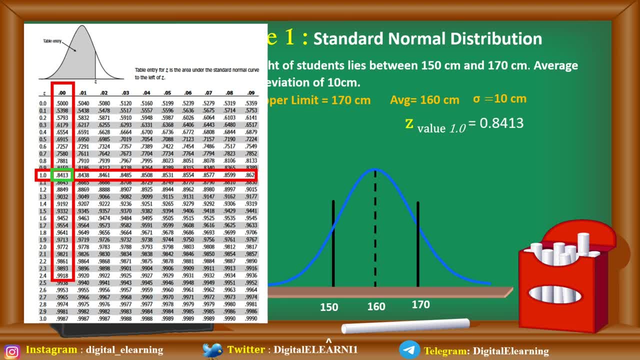 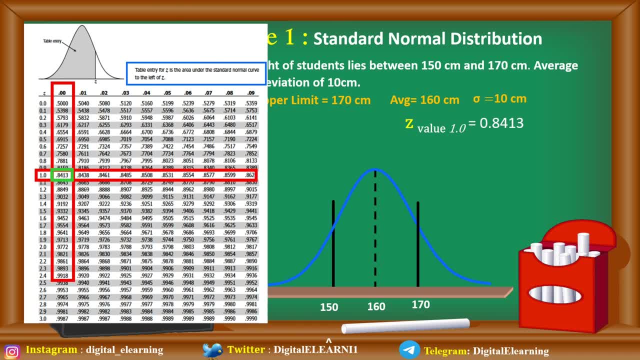 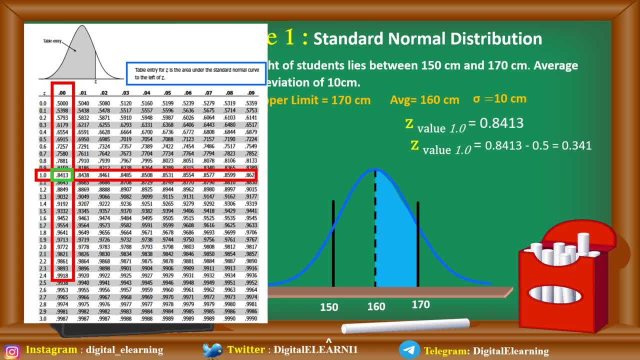 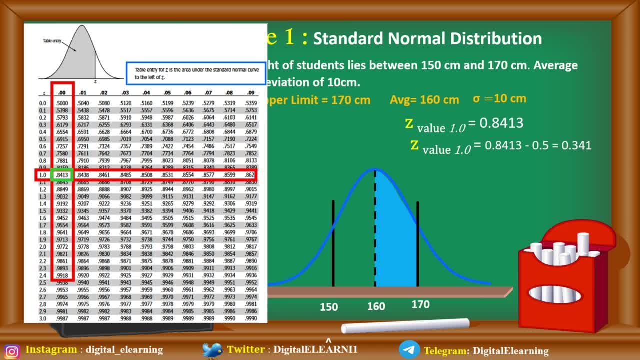 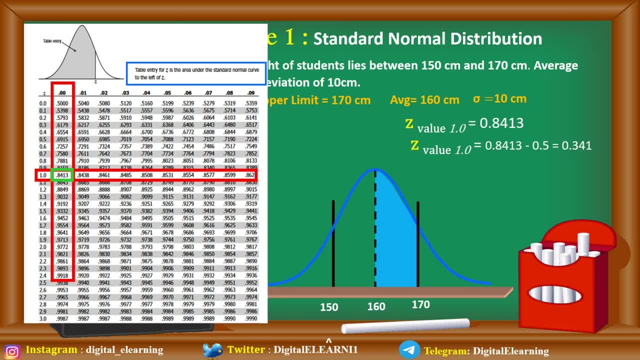 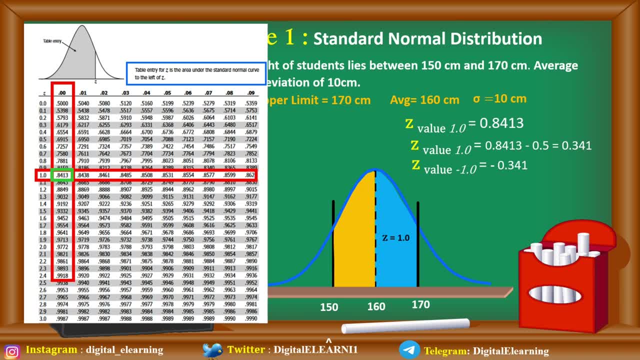 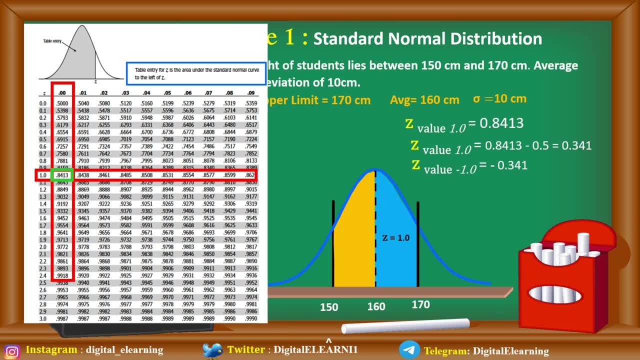 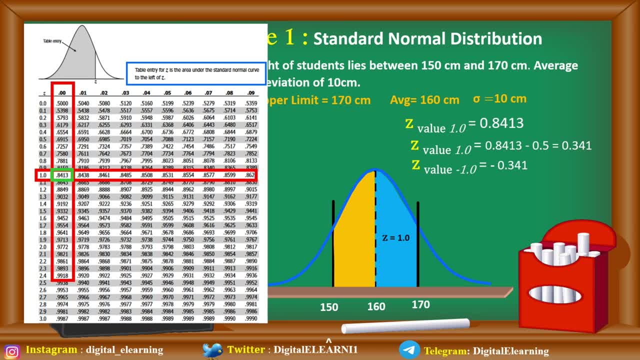 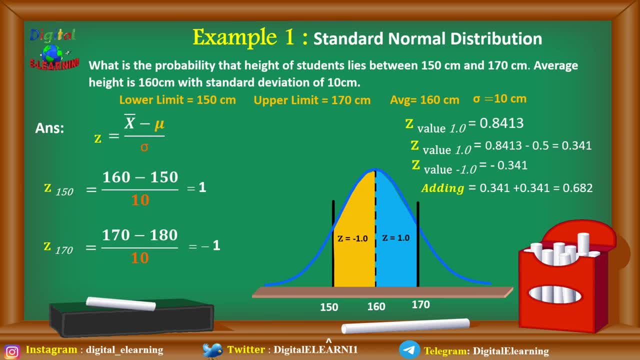 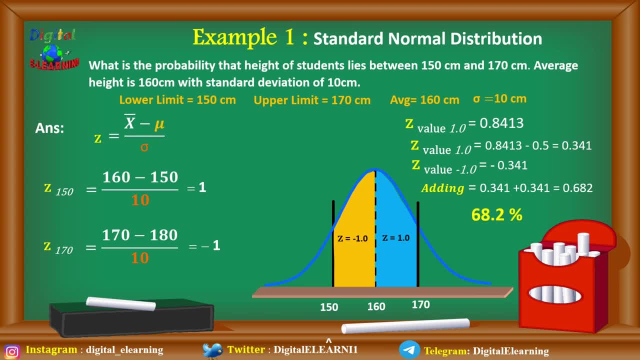 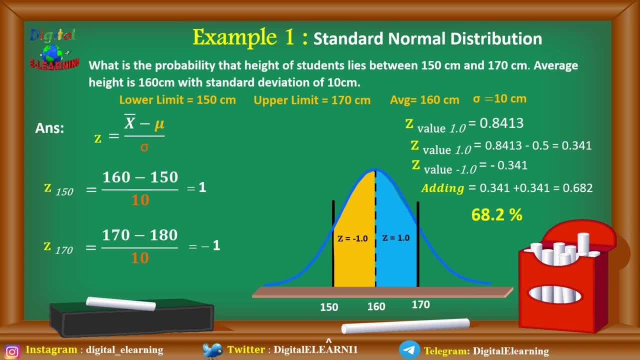 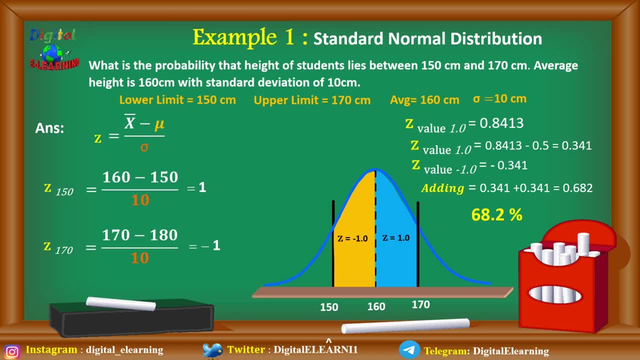 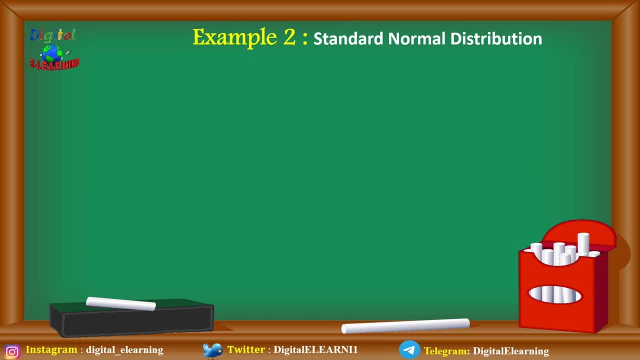 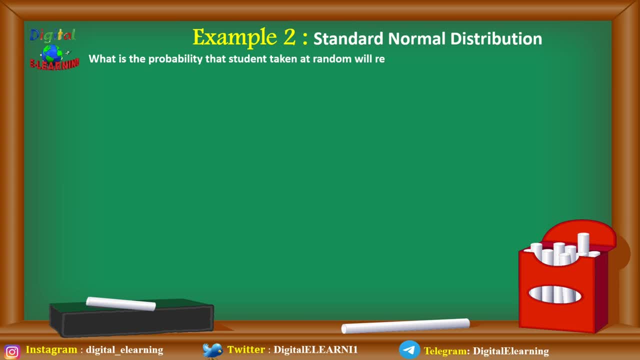 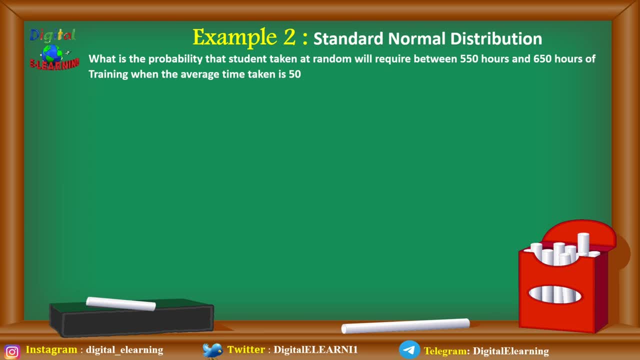 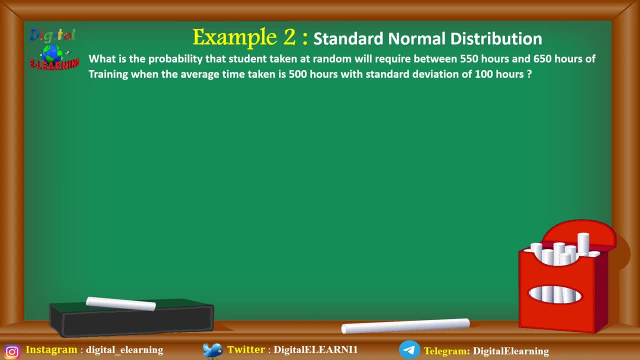 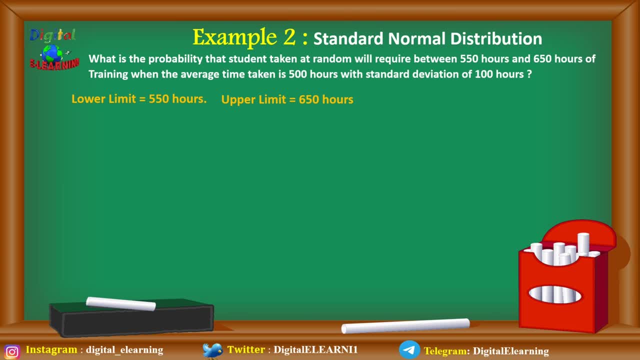 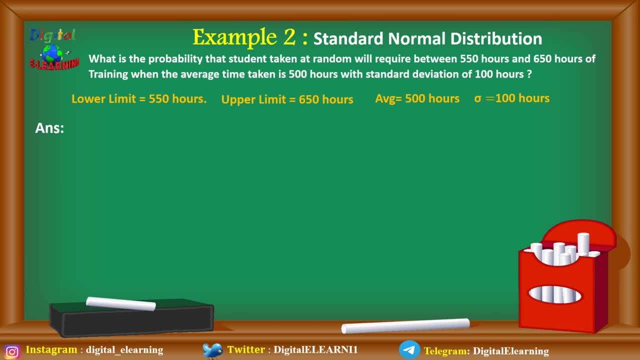 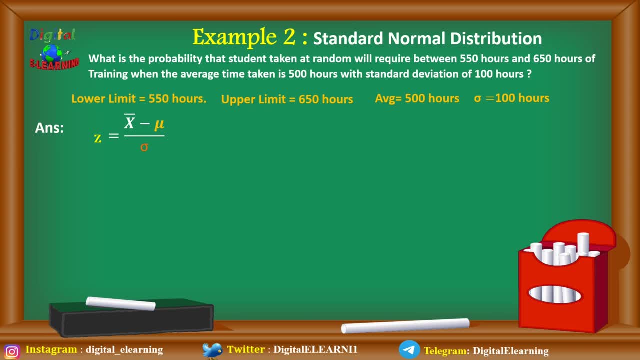 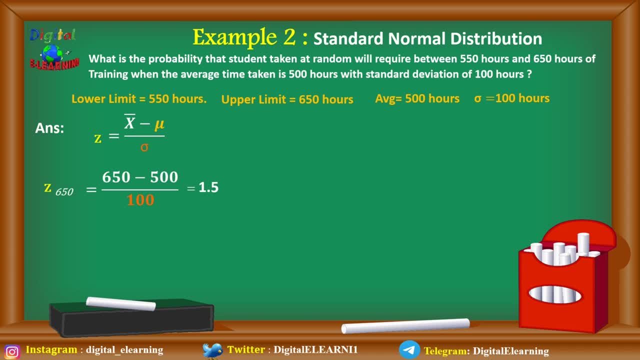 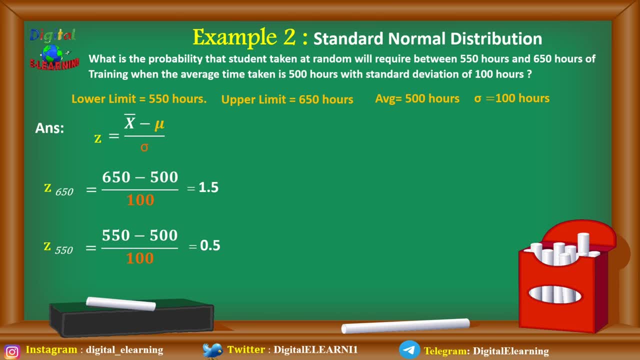 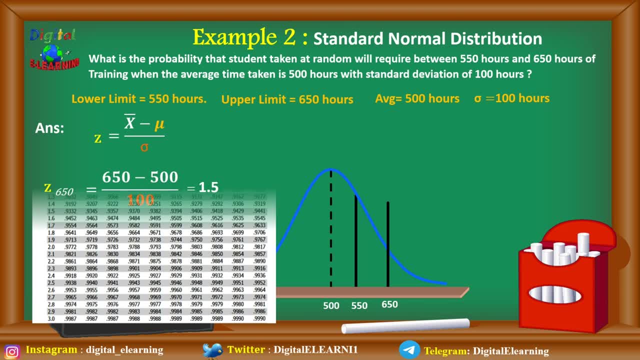 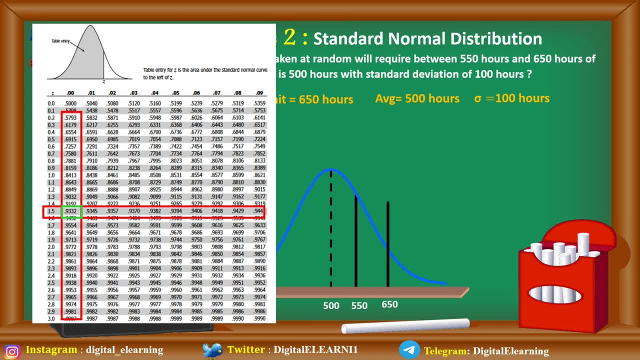 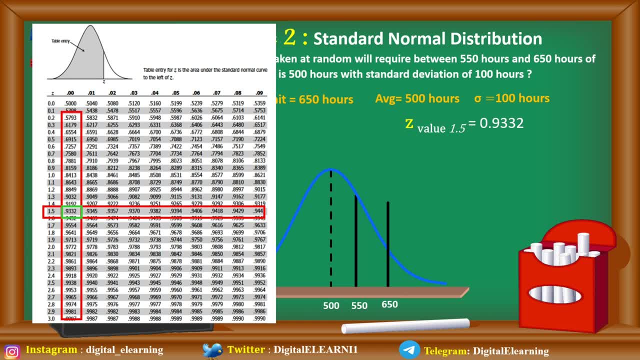 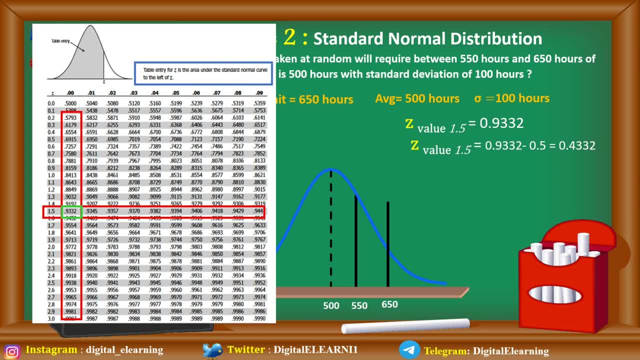 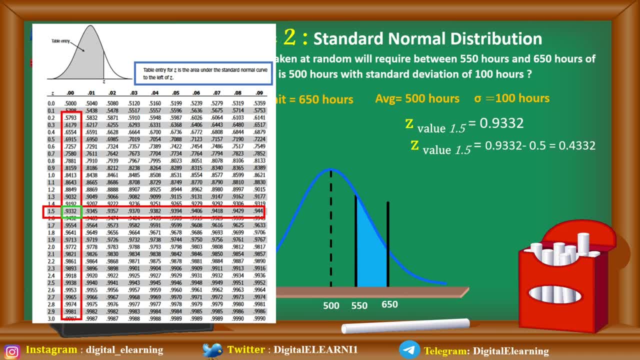 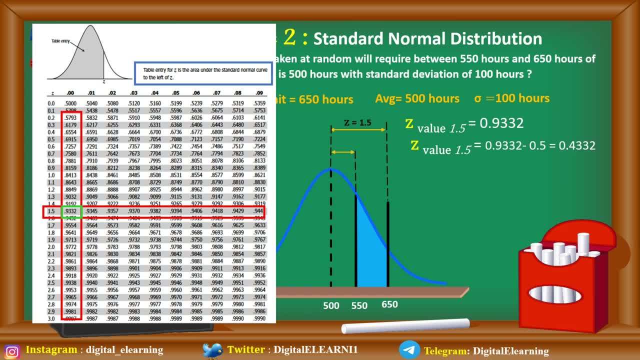 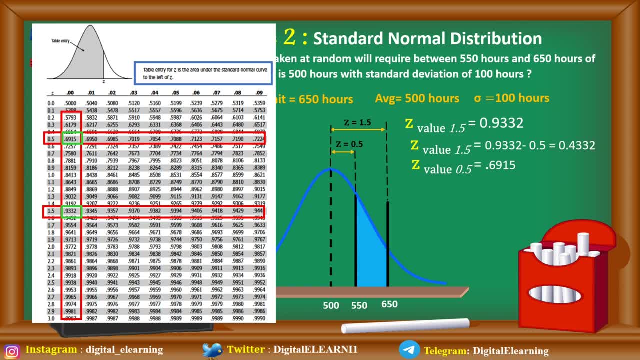 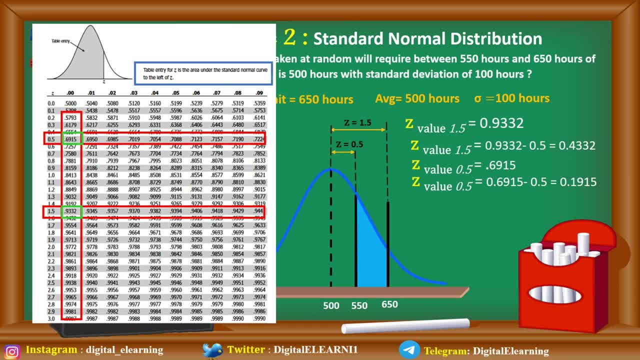 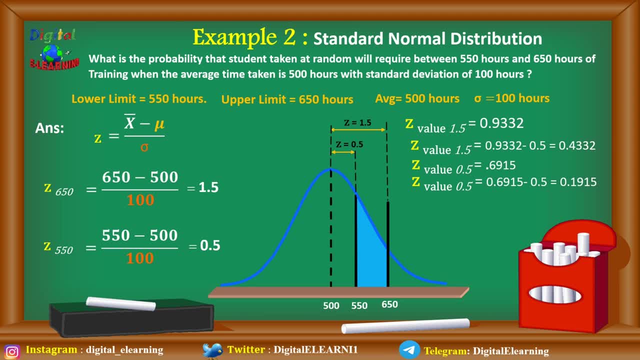 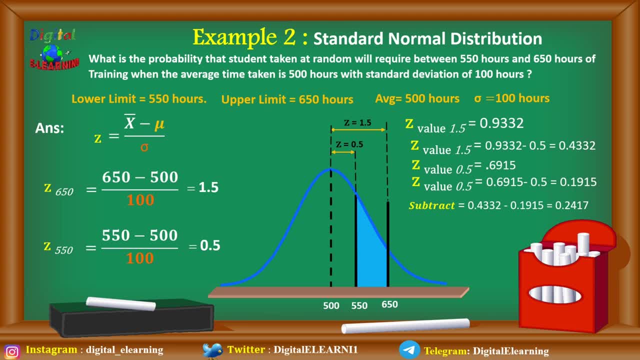 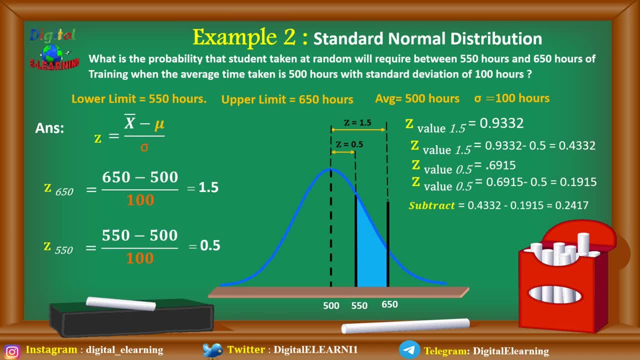 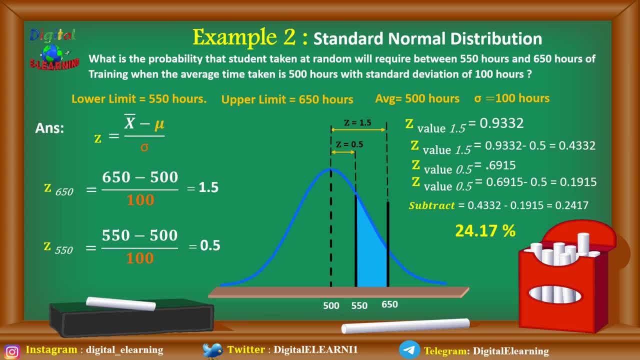 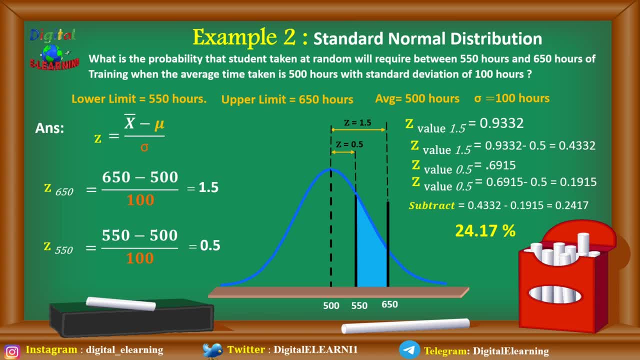 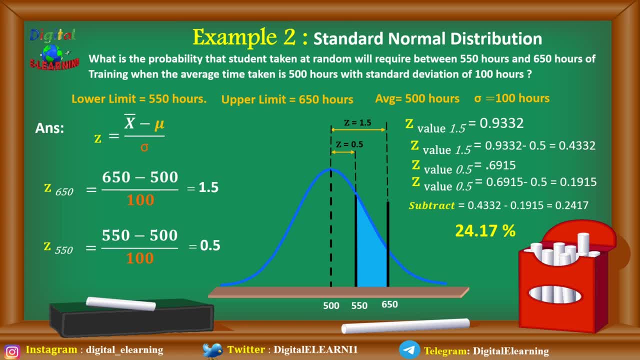 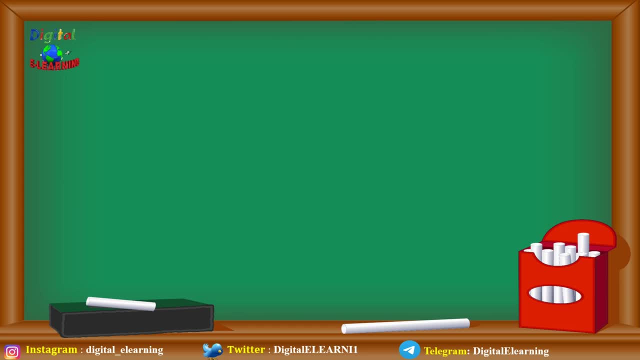 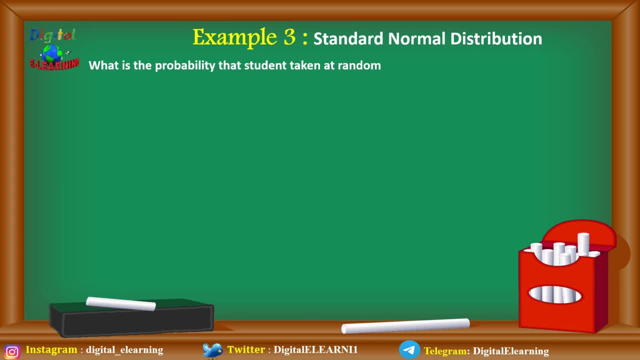 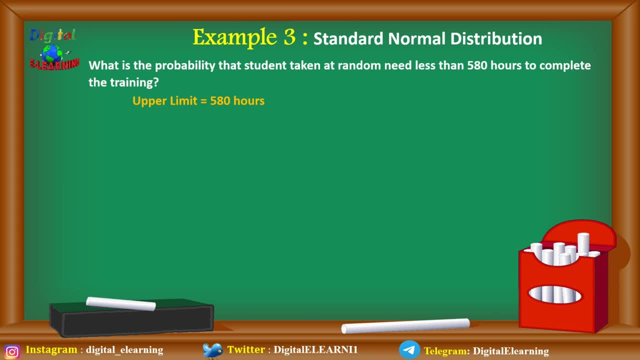 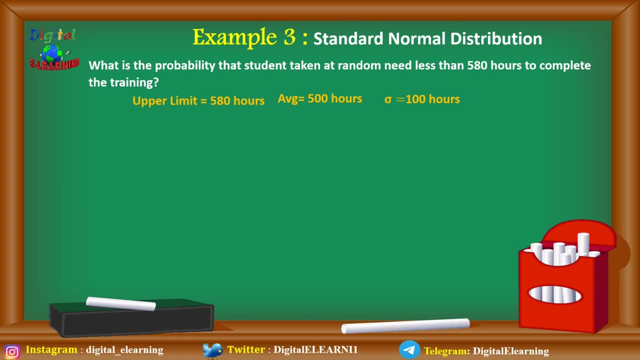 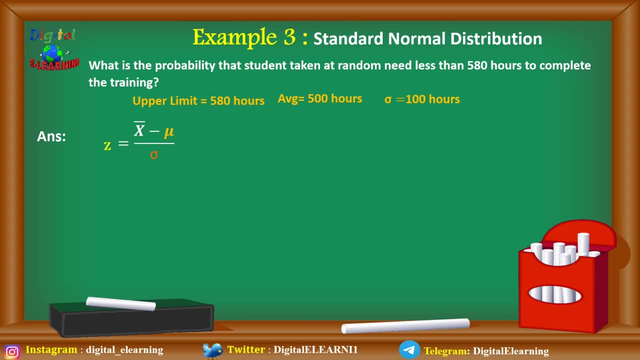 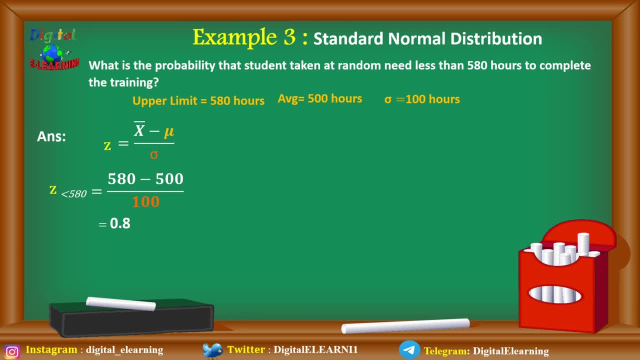 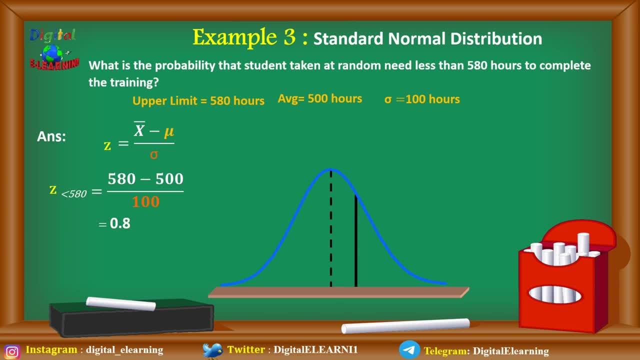 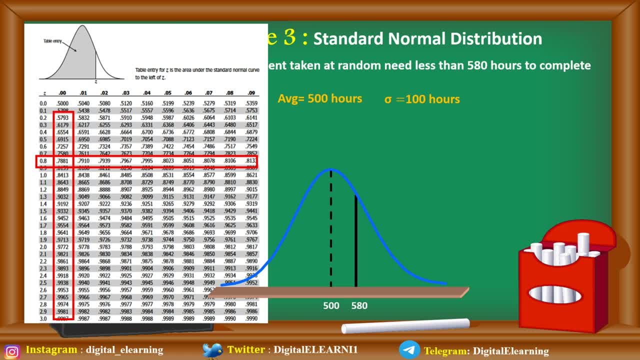 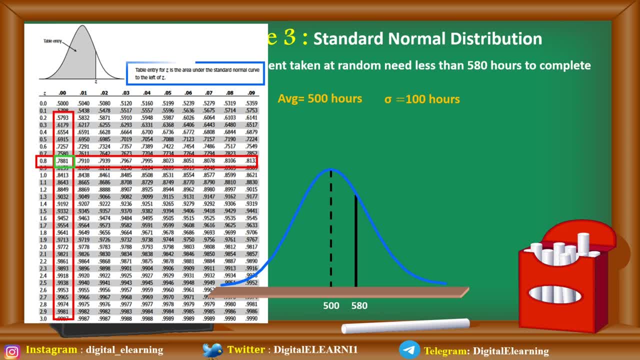 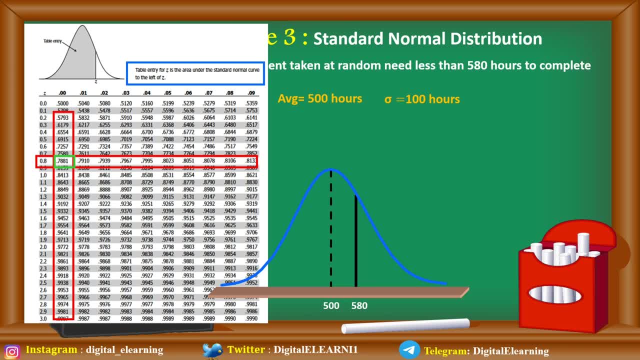 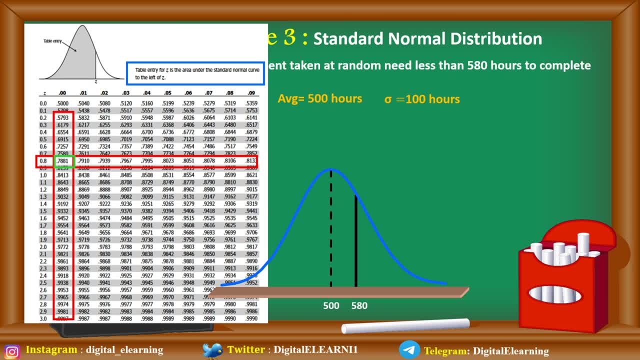 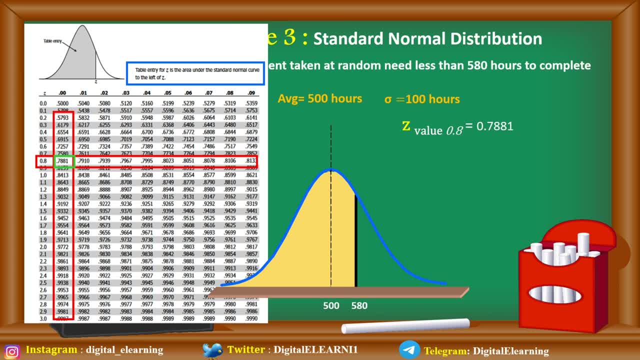 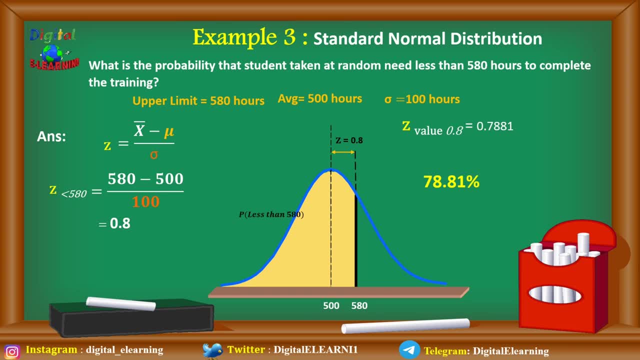 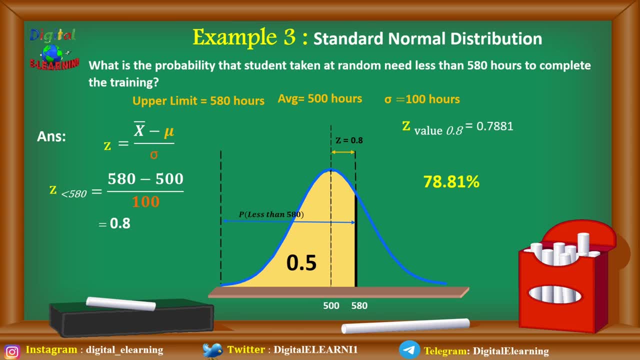 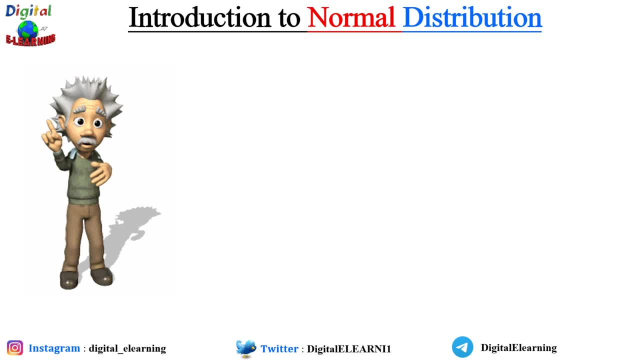 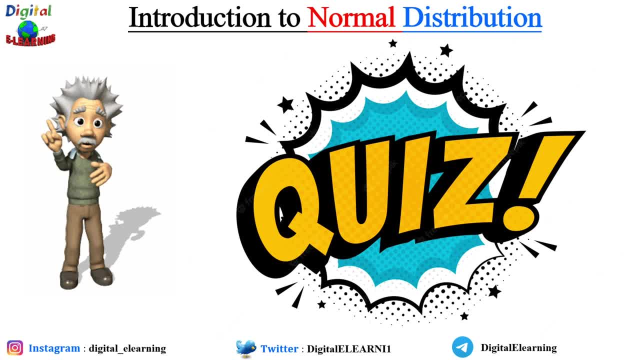 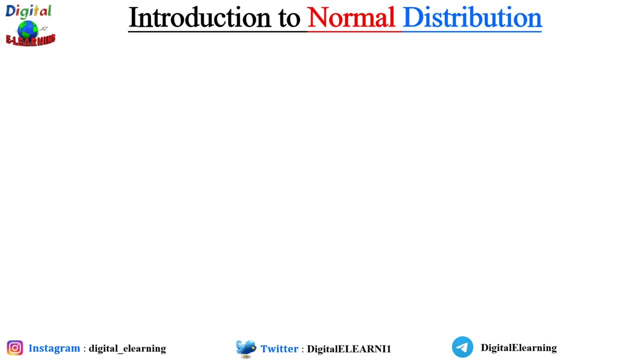 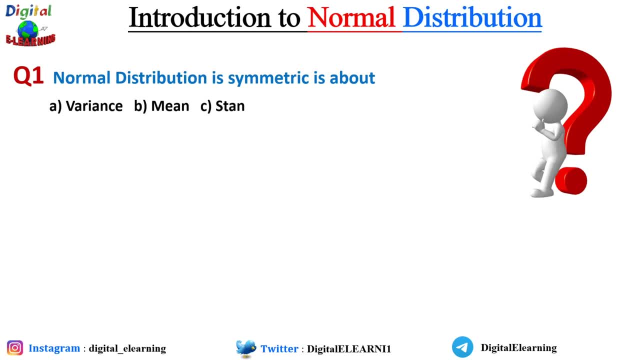 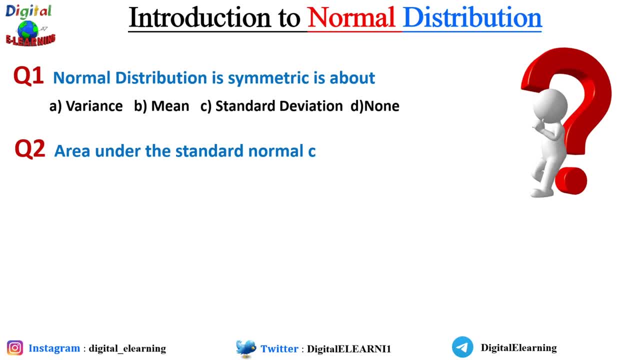 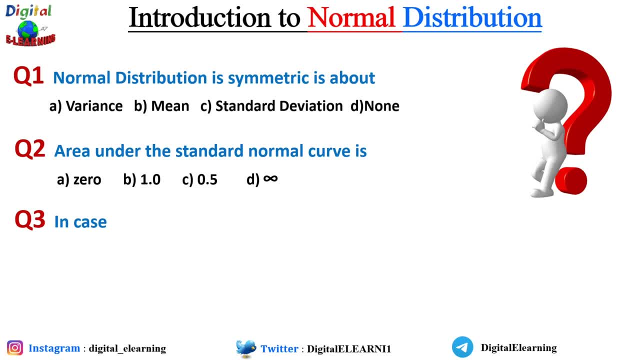 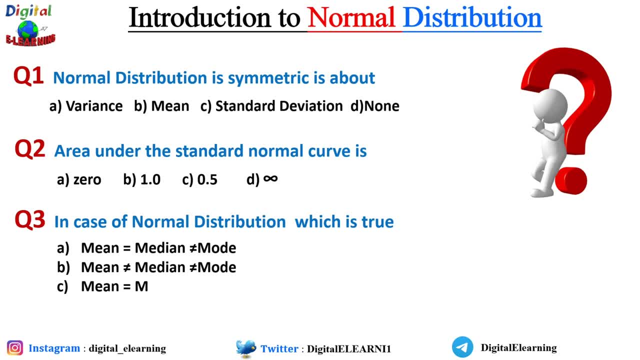 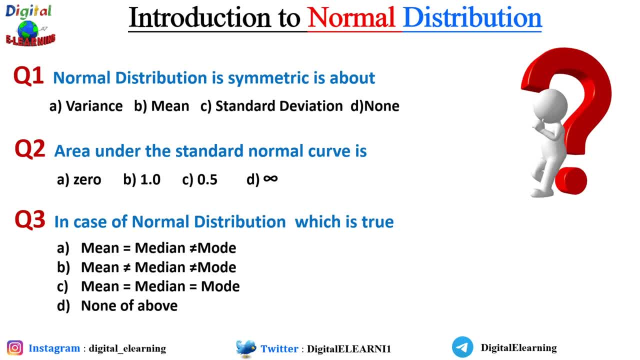 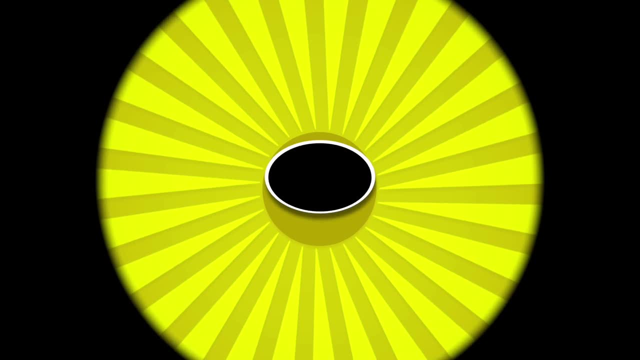 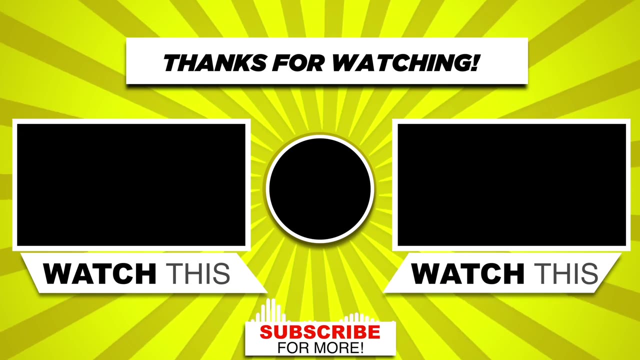 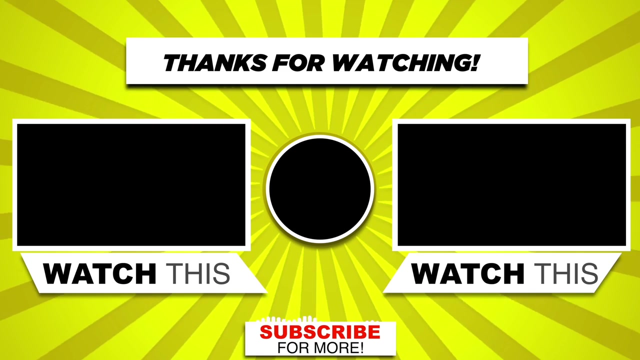 The shaded area under the curve here is the probability that X lies between A and B. The shaded area under the curve here is the probability that X lies between A and B. 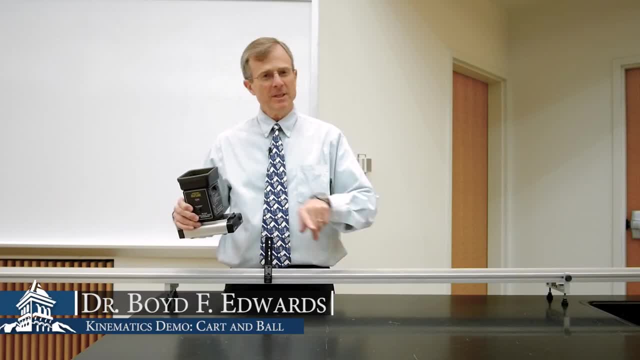 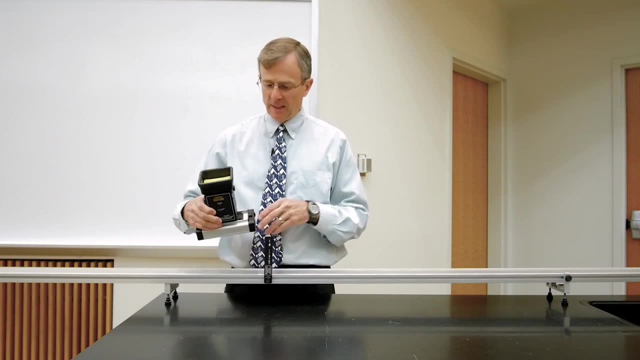 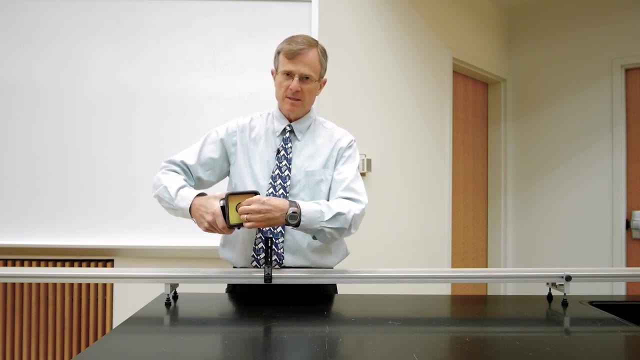 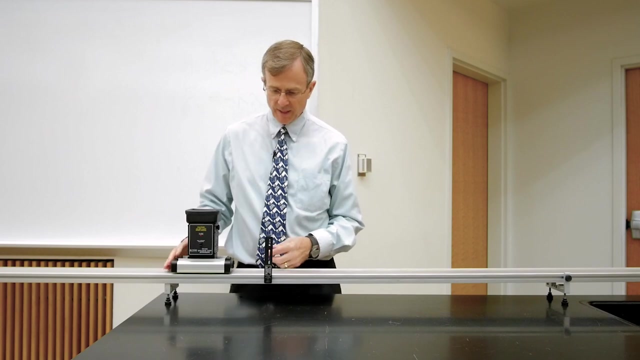 This is a demonstration of the independence of motion in the X and the Y directions. What I have here is a cart that moves along the track and a ball with a plunger, And when I depress the plunger, then the ball is released and the plunger activates when 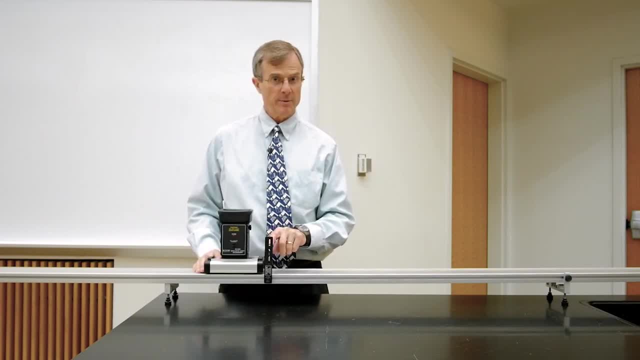 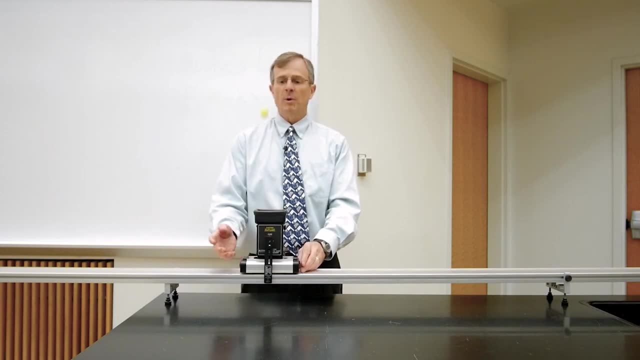 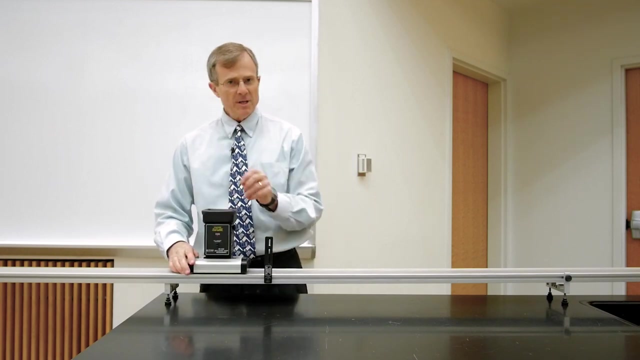 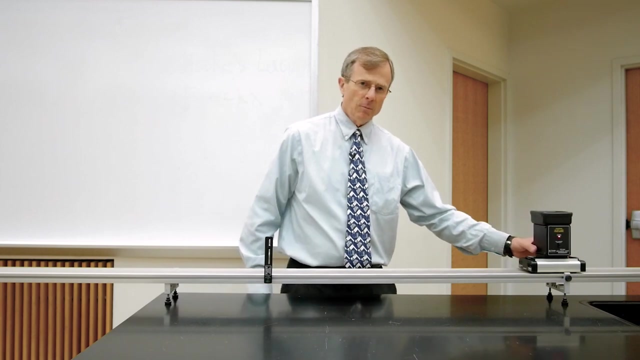 this sensor passes a little metallic strip right here, So if the cart isn't moving, then the ball goes straight up and down and comes right back down to where it started. If I depress it again and give it a little bit of momentum, then what happens is the.